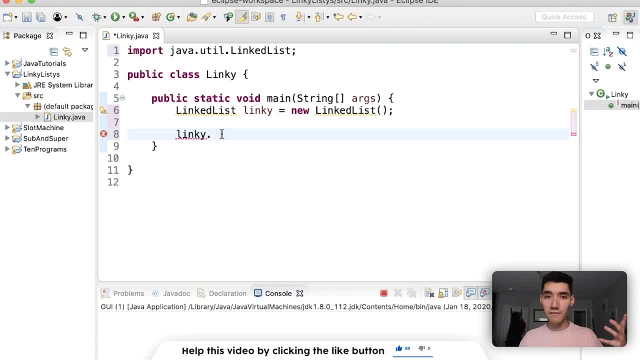 You can iterate through it. You can see if it's empty. It's a very flexible data structure. It's called a linked list because each value in the list knows the front and next element which makes it really flexible of a data structure. 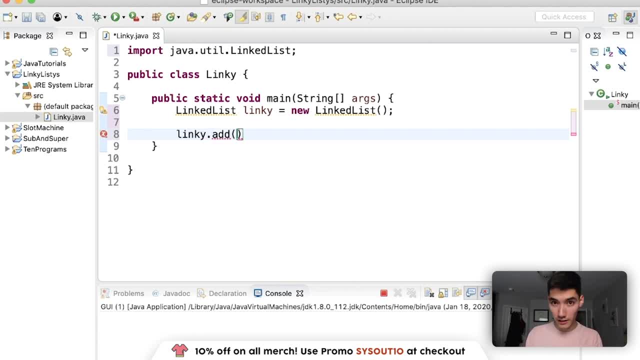 It's super awesome, So let's add some stuff to it. Let's say: we've got strings, We've got Rob, We've got me. Put Alex in here, We've got you. Let me guess what your name is: Jose. 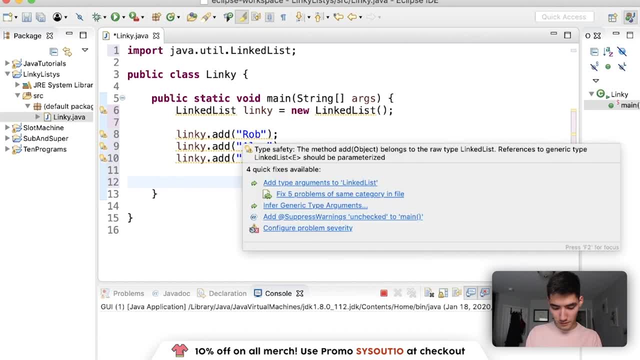 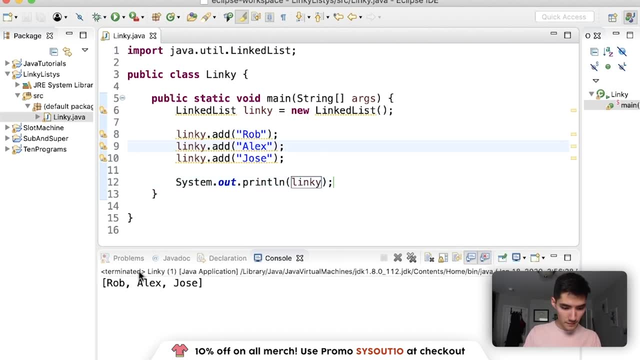 Your name is Jose and we are going to print you out. Let's print out everything in the linked list data structure. We've got Rob, Alex, Jose, which is the order that we added, So it keeps the order. If we want to remove from a linked list, we can do this. 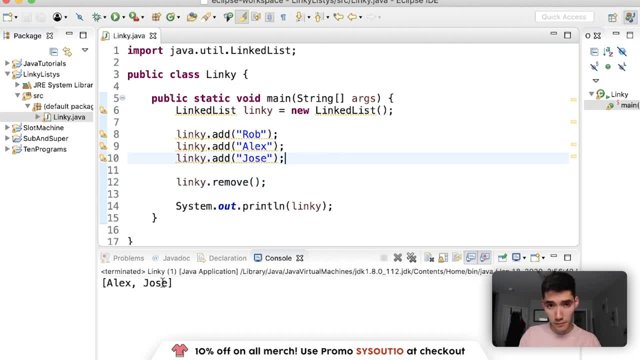 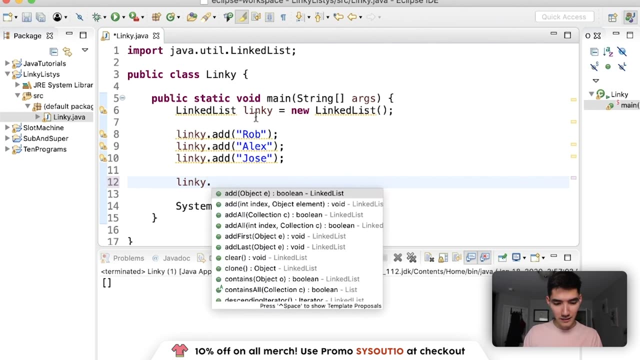 Remove, Boom And it removes from the front. We can clear everybody from the list like this: Clear Everyone is gone. If this seems a little fast, don't worry, because all I'm doing is typing the name of the linked list and doing a dot. 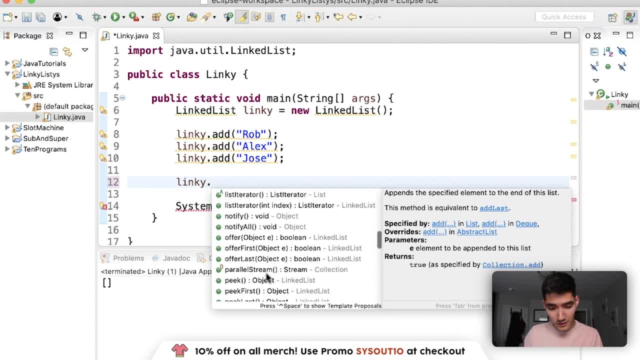 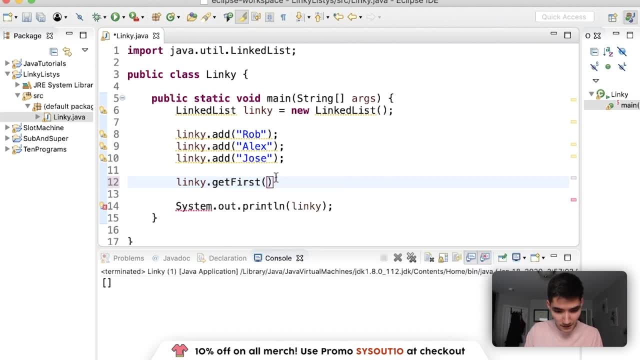 And these are all the methods that that linked list can do. So I'm literally just like picking methods from here. I could click it and do one like: get first, Get first, Let's see what that does. It gets the first element, but we're still printing the whole thing. 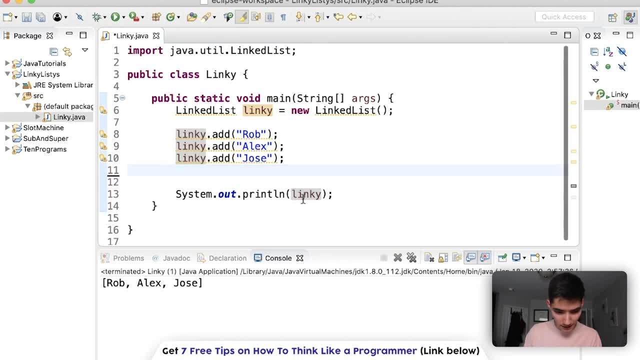 So obviously it's not going to show up, So let's put that in here instead. We'll get the first, and that is Rob. We can get the last. We can do all sorts of stuff with the linked list. We can even do integers in here. objects. 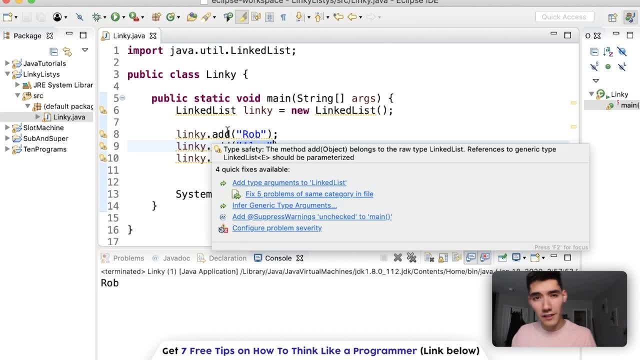 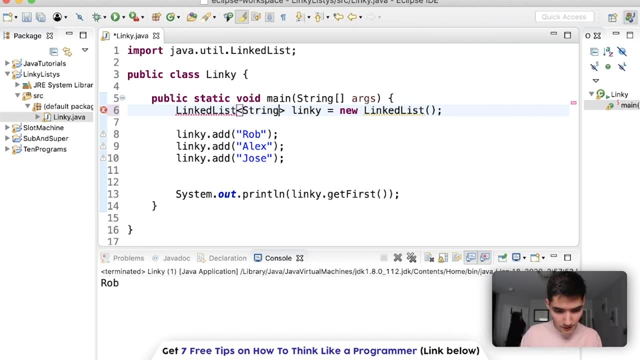 We're really just scratching the surface. It's good practice. We see a bunch of yellow underlines here- because it wants us to do the good practice thing And put the type of the elements inside of little alligators here And those underlines go away. 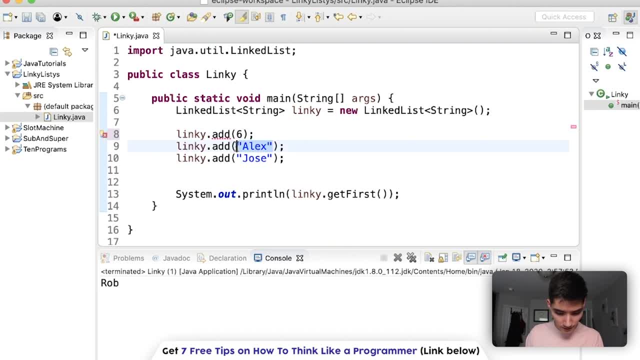 Let's start over. Let's start over and do some numbers. So we've got 6,, 78, and 1.. These are red because it's like: well, you told us it was a string, But it's actually an int. 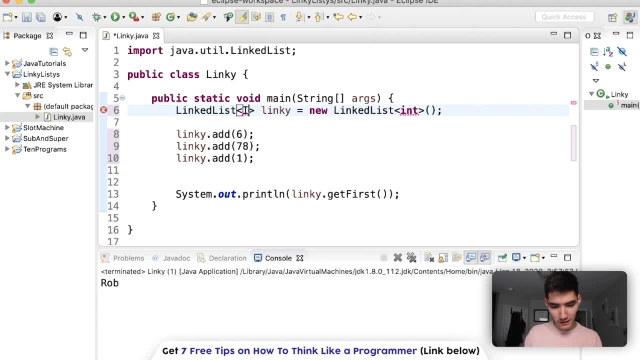 And now it's like we can't put primitive types in here. Alex, It has to be the capital one. Okay, Save and run. And now it just works with integers. So let's try to iterate through these And say we want to get. 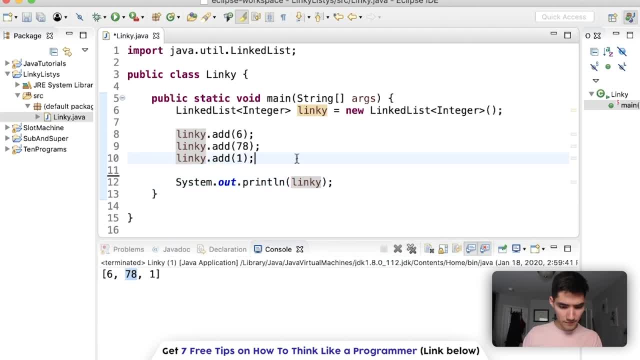 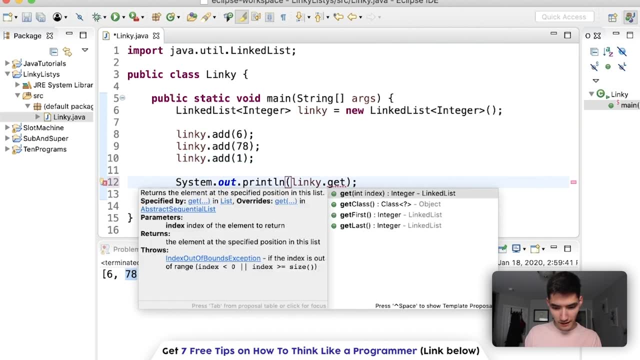 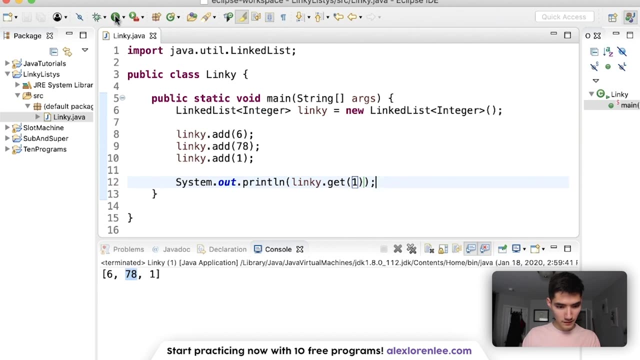 78.. How do we get just 78 and not the entire linked list? Well, we can do that like this: Gets 1 at a certain index. We know indexes start at 0. So 78 would be 1. Boom. 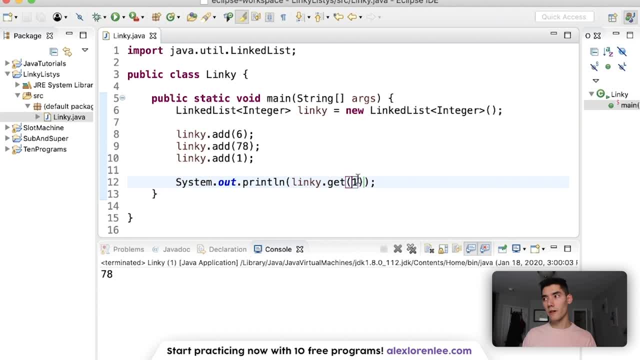 And that's how we get 78. But what if you don't know the index? Or what if you have 100 elements in your linked list and you don't want to worry about the exact index? Well, you can iterate through them using an iterator. object: 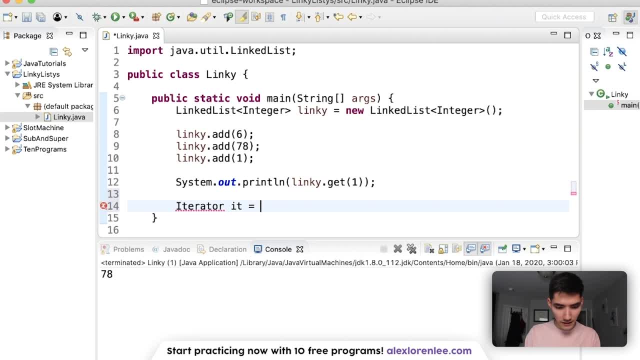 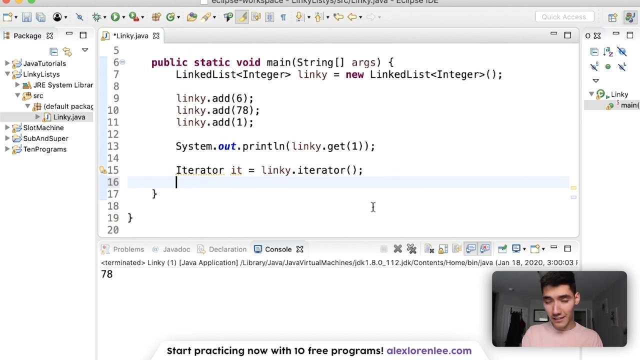 So we'll just do the same thing, But make an iterator instead Iterator. Pop that in here using javautil And instead of making a new iterator, we're going to use the linked list iterator by doing linkyiterator. Boom, Now I can iterate through it and get the 78 that we want. 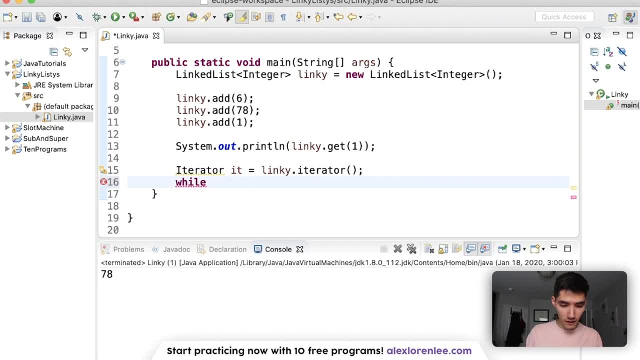 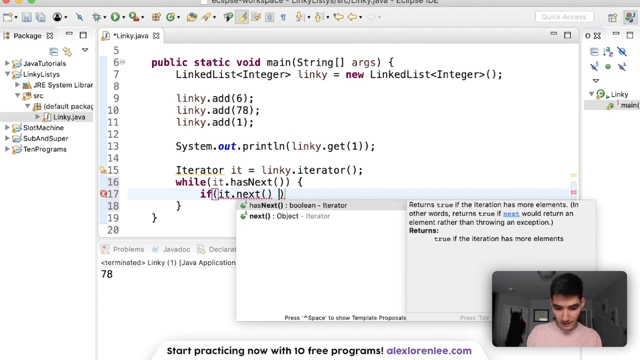 To use an iterator. you usually throw it in a while loop And you do while the iterator has something. next, Then we will do stuff And say: if that thing, if itnext is equal to 78,, then we will print out. 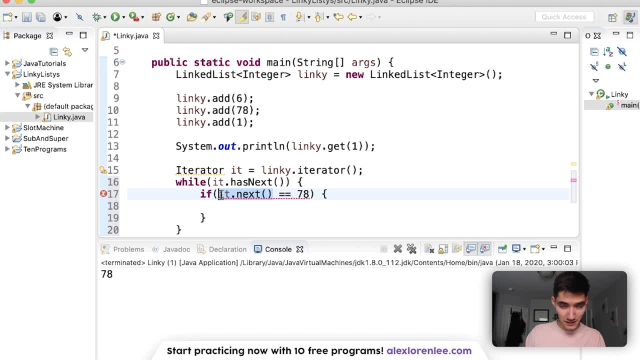 And it's saying: we need to cast this Because this returns an object and this is an integer. Maybe we can cast it like this: Ints. Yeah, So we'll try that And we can print. We found 78. Boom. 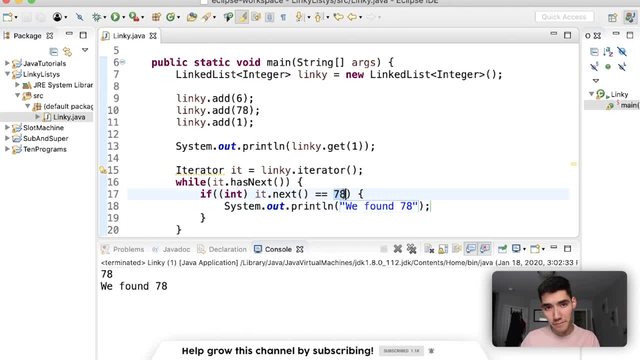 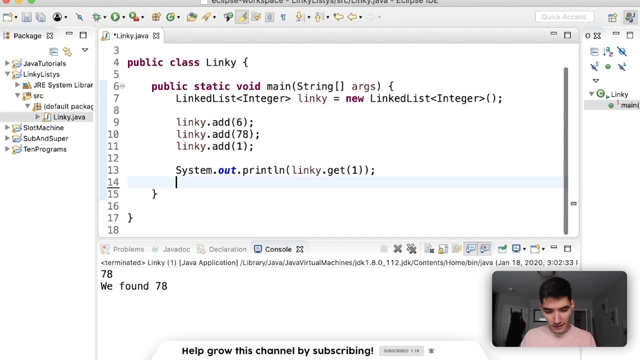 Like that And we can run code based on the specific element. So that was super quick. on how to use the important things of a linked list, There's also a few other ones like Is empty, And there really there's just so many.